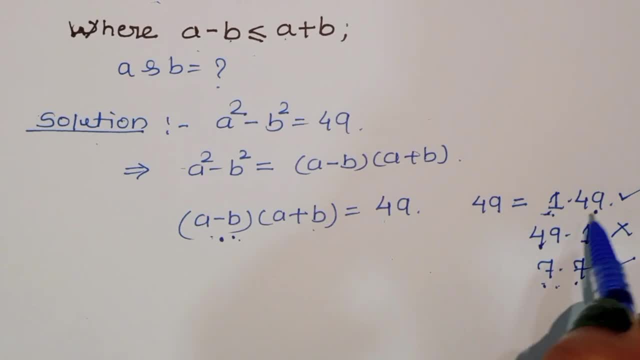 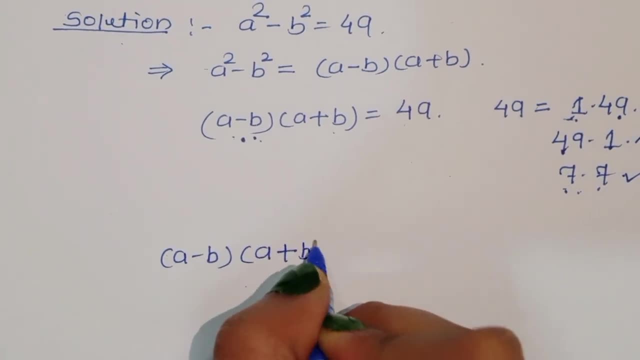 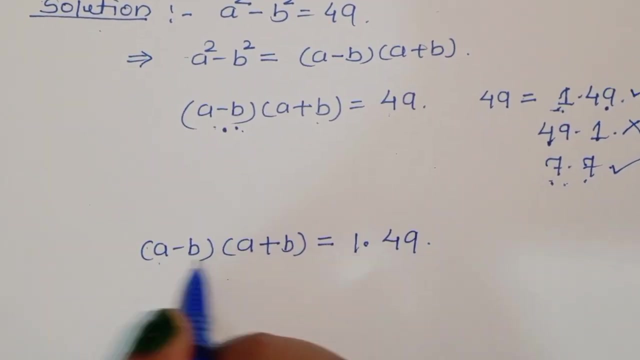 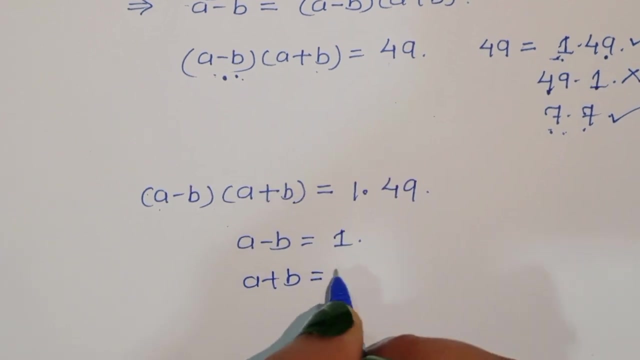 So this is also satisfied. So first we are taking first term. That is a minus b times a plus b is equal to 1 times 49. Now here, comparing a minus b is equal to 1 and a plus b is equal to 49.. 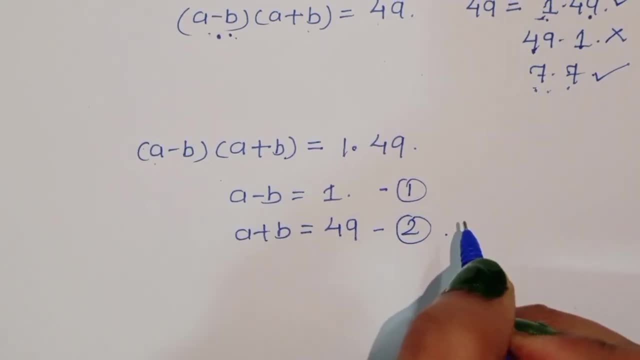 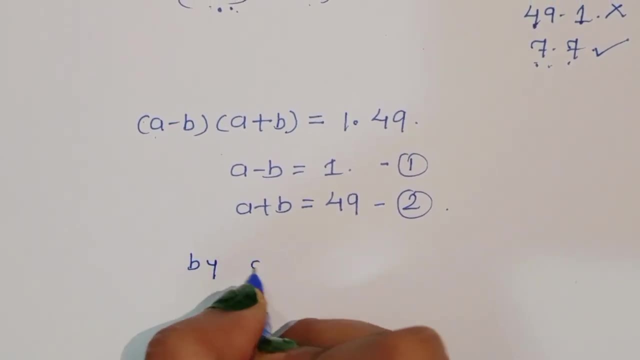 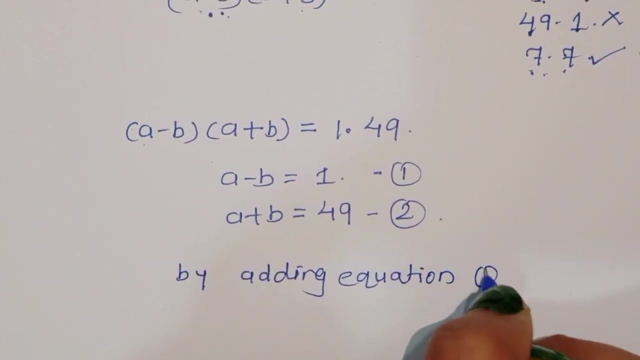 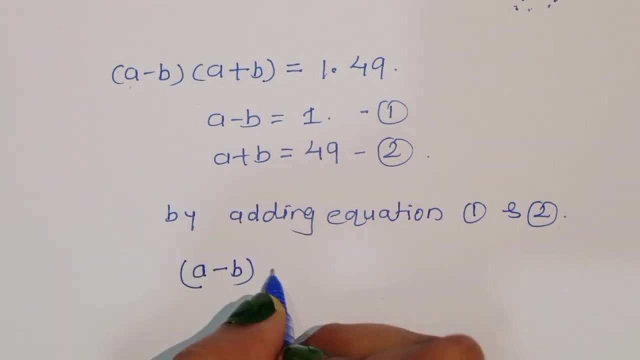 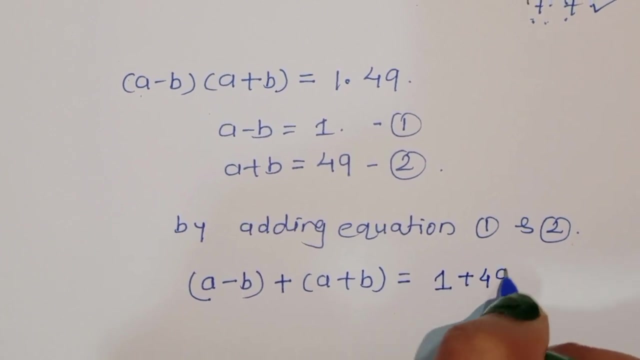 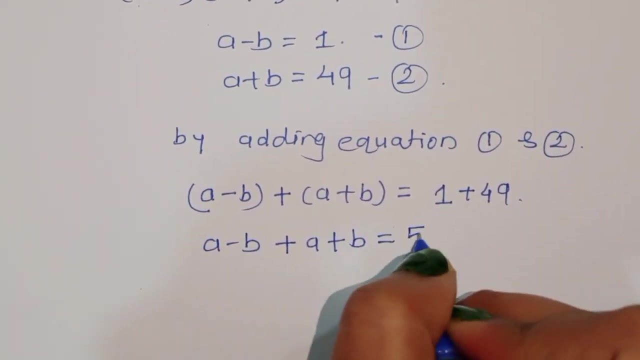 This is equation 1 and this is 2.. Now we can here add: By adding Equation 1 and 2, we will get a minus b plus a plus b is equal to 1 plus 49.. Now a minus b plus a plus b is equal to 1 plus 49 is equal to 50.. 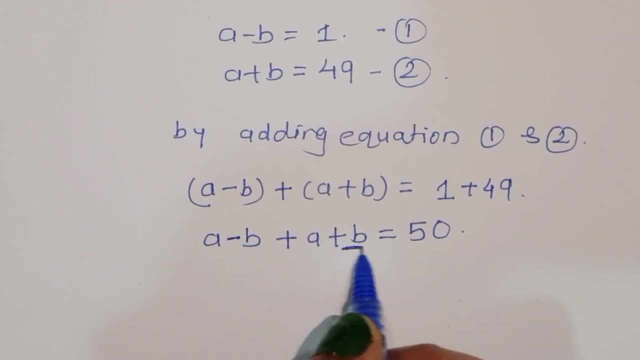 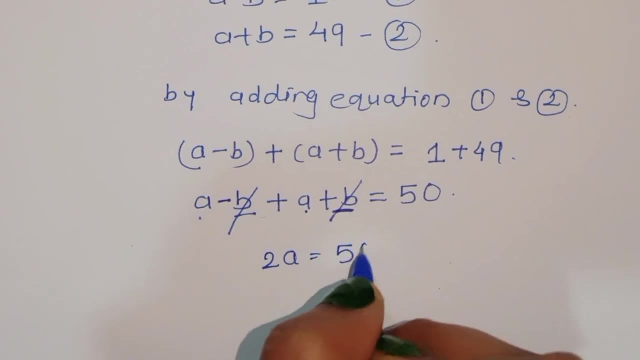 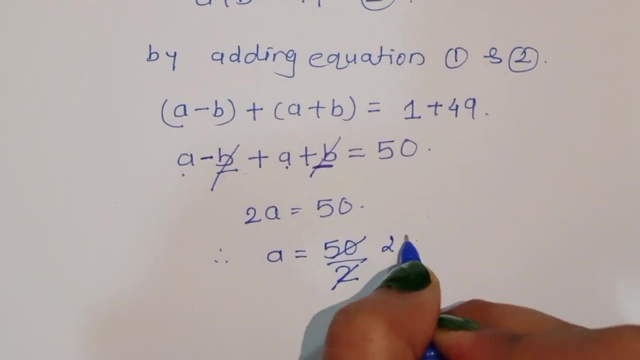 Now you can see here: minus b and plus b. This will cancel A. plus a, 2a is equal to 50. Therefore, we can write: a is equal to 50 divided by 2. 25.. Right, So we got here. value of a is equal to 25.. 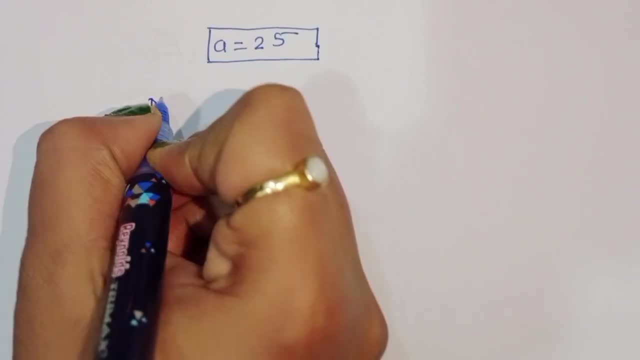 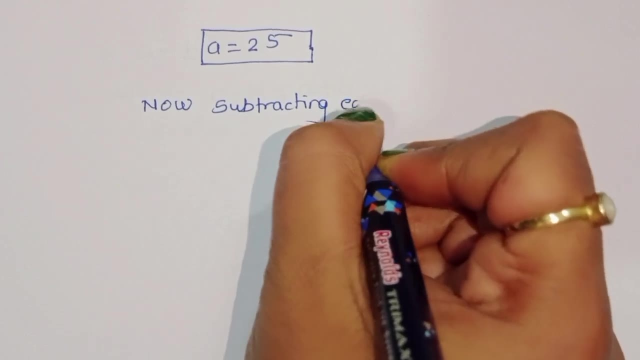 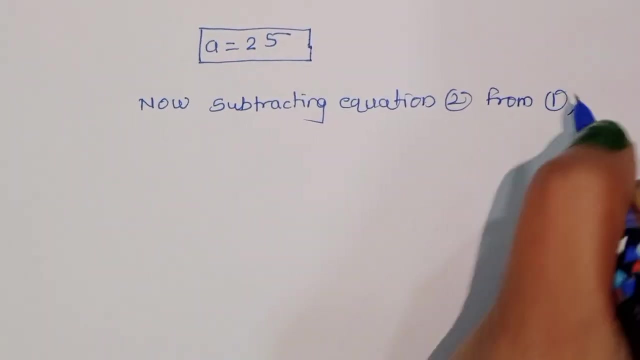 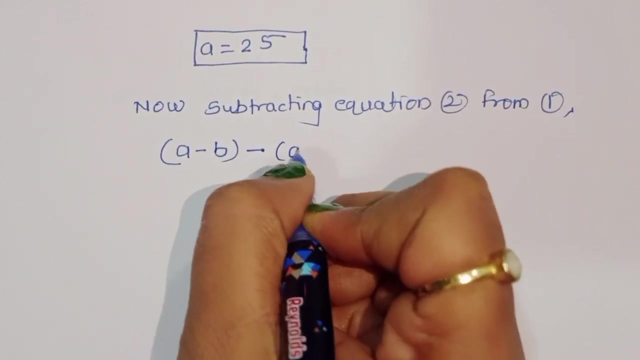 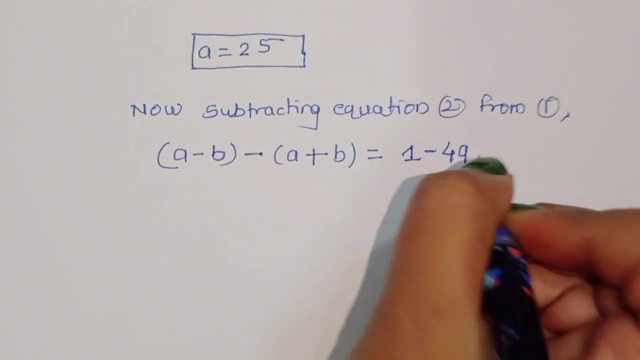 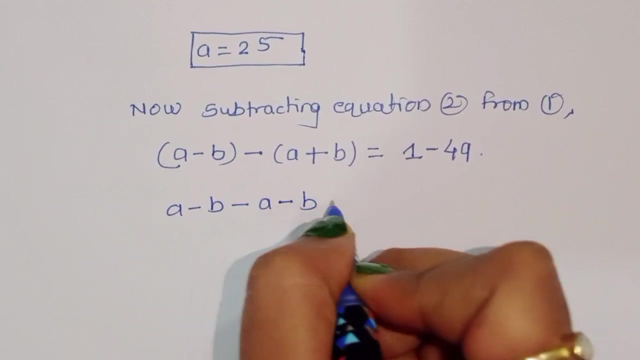 Now, Now. Now, Subtracting Equation 2 from 1.. Then we will get a minus b minus a plus b is equal to 1 minus 49.. Now, a minus b minus a minus b is equal to 1 minus 49.. 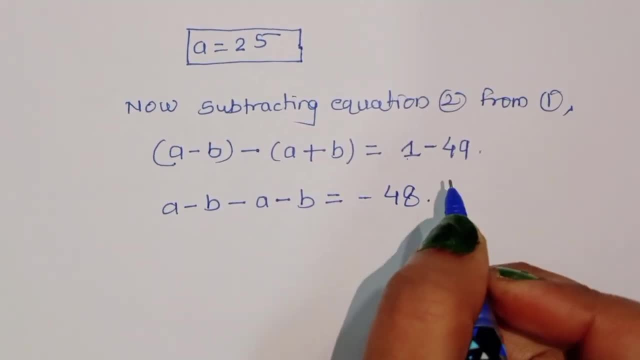 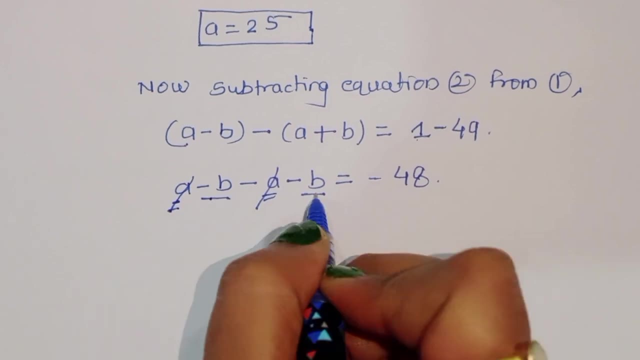 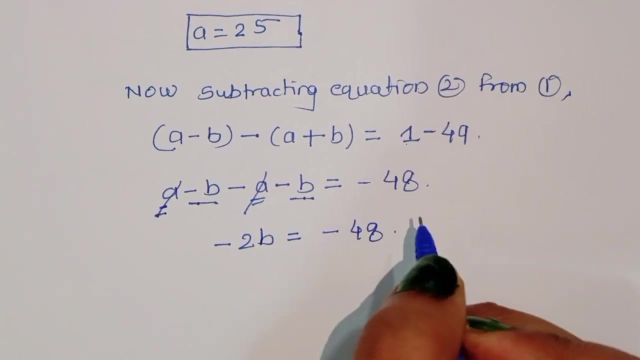 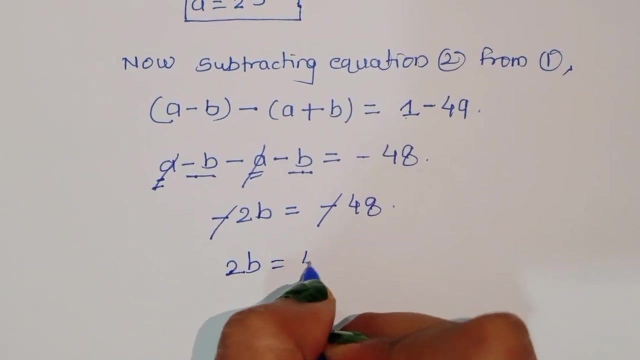 That is 48.. Now minus b minus b, plus a minus a. So this will cancel here. minus b minus b minus 2b is equal to minus 48.. Right Minus is cancelled from both side. Now we can write: 2b is equal to 48.. 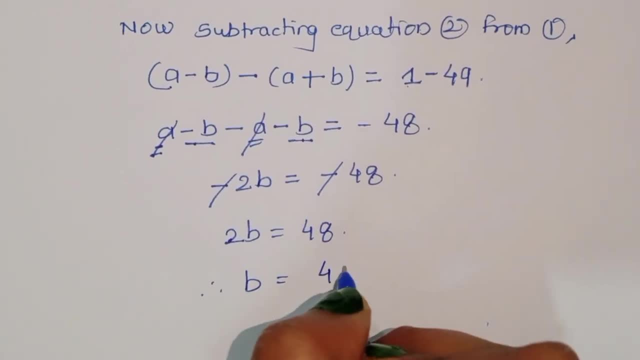 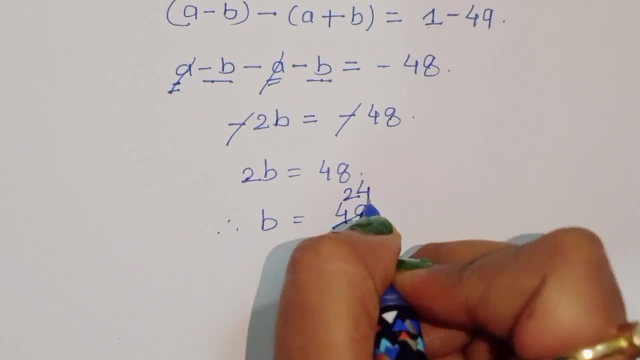 Therefore, b is equal to 48.. Right Now, 2B is equal to 4.. Levi by 1 divided by 2, 2, 2 is 4, 2, 4 is 8.. b is equal to 24.. 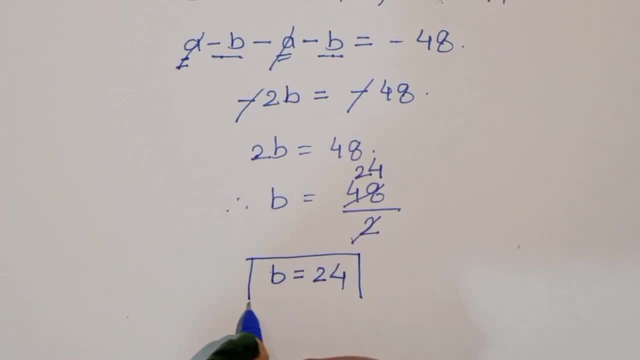 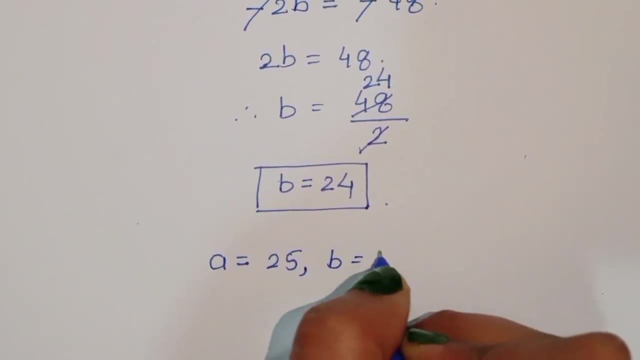 This is the value of b. So we got a 2 value. A is equal to 25 and b is equal to 24 from first factor. Now we are using a second factor, That is b minus a minus b is equal to 24.. 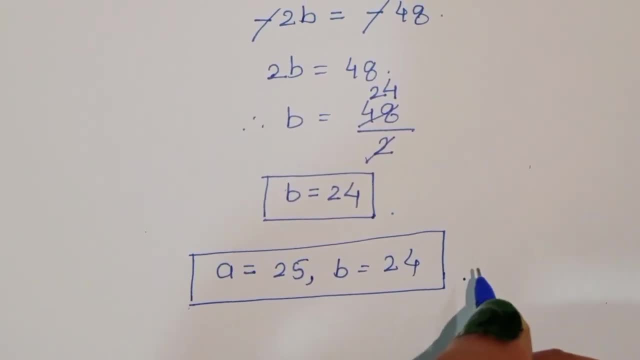 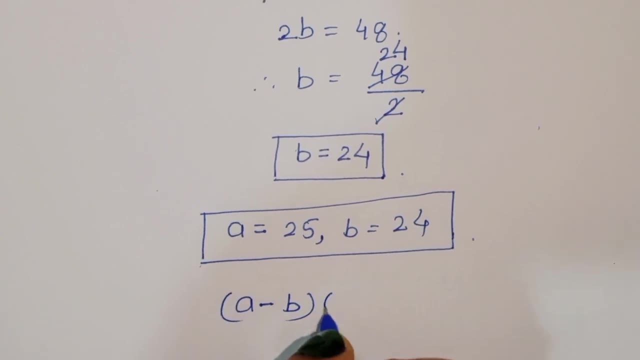 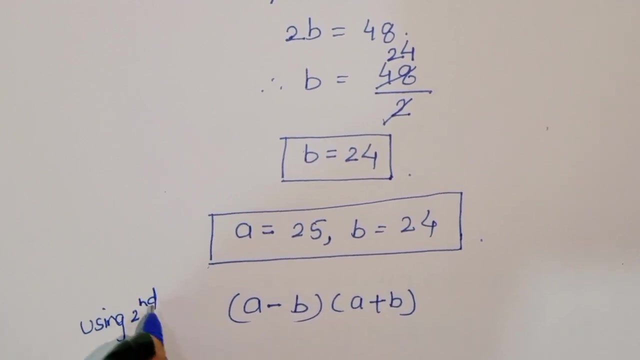 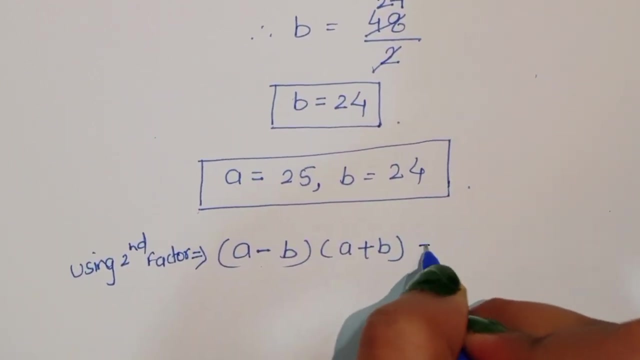 Now we are using a second factor, that is a minus b. minus b is equal to 26. Right times a plus b. this is using second factor. using second factor, a minus b. a plus b is equal to 7 times 7. right, because a minus b. 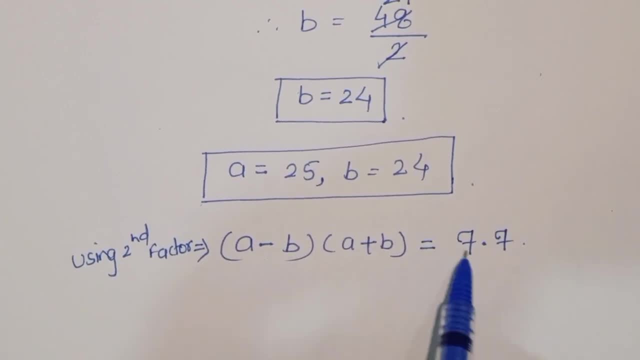 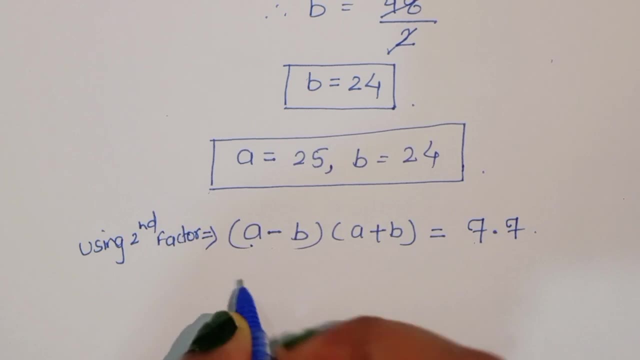 is equal to a plus b here a minus b 7 and a plus b 7, and this is given in condition, that is a minus b equal to a plus b. so we can write this, comparing this, both terms we can write- a minus b is equal to. 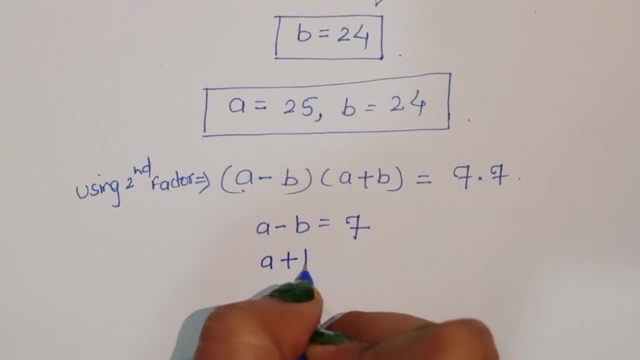 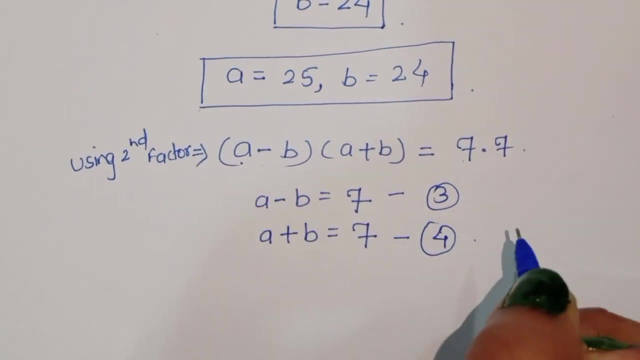 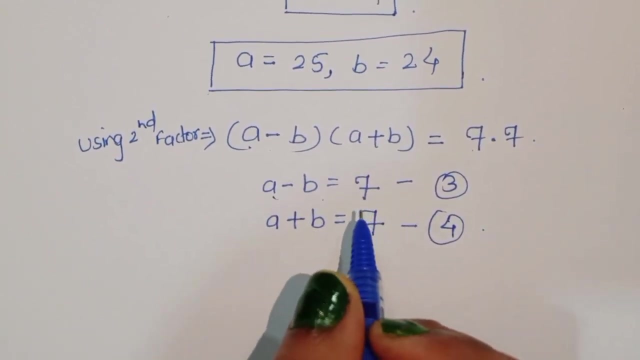 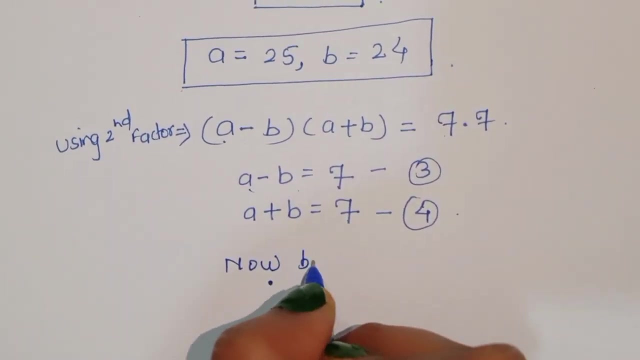 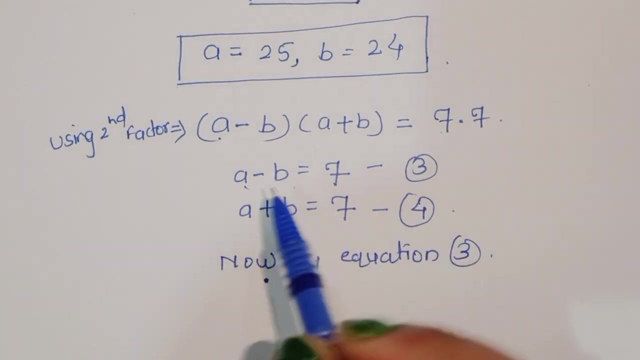 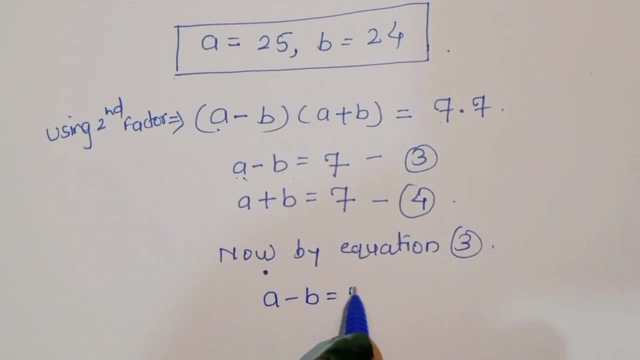 7 and a plus b is equal to 7. this is equation 3 and this is equation 4. now again we can write here a minus b equal to 7 and a plus b equal to 7. therefore we can write here by equation 3 what is given in equation 3: a minus b is equal to 7. right? so a minus b is equal to 7. 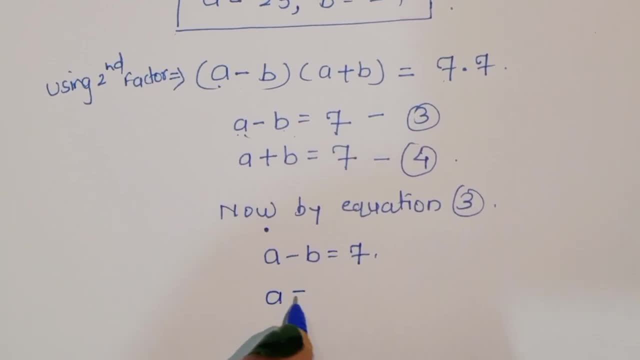 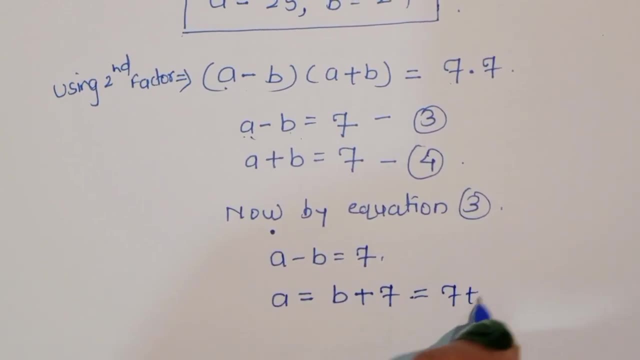 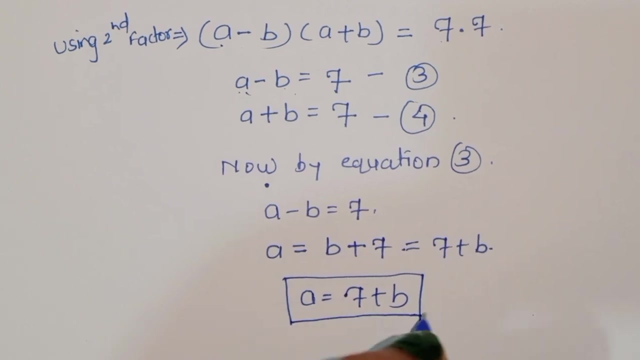 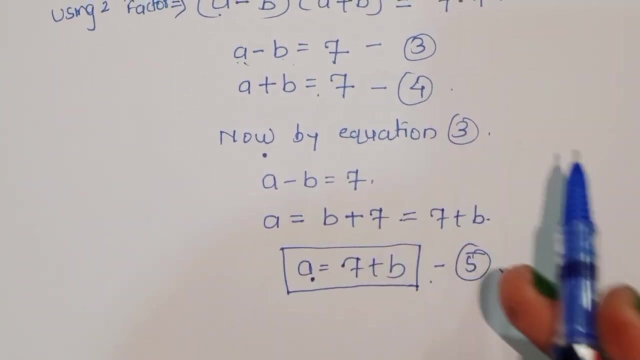 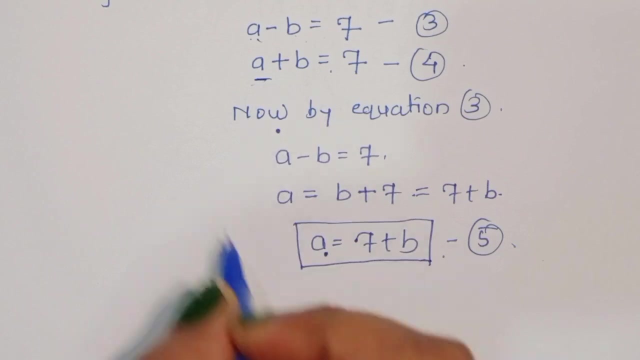 so we can write here: a is equal to b plus 7, right, or 7 plus b. so this is the value of a, that is 7 plus b. now this is equation number 5. now this value we have to substitute here in this equation now, then we will get 7. this is a plus b is equal to 7. now, value of a.